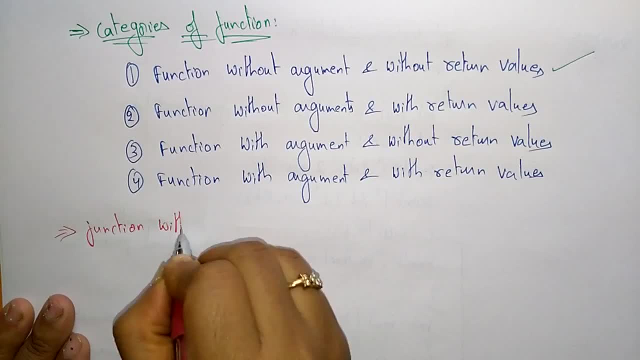 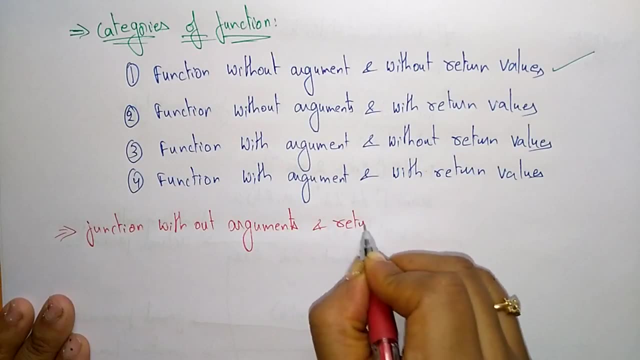 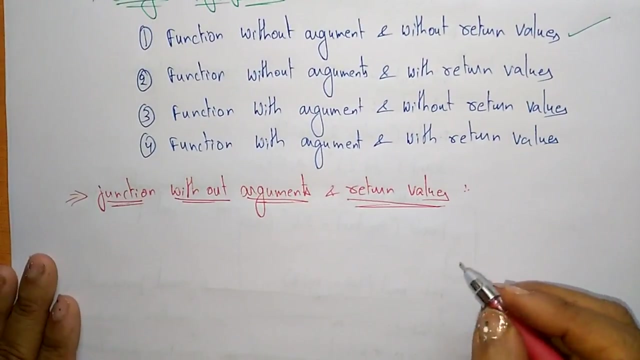 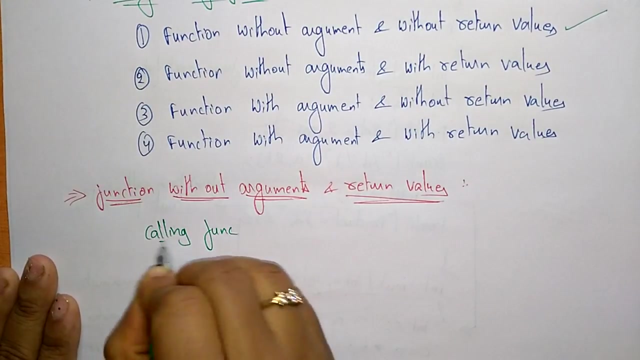 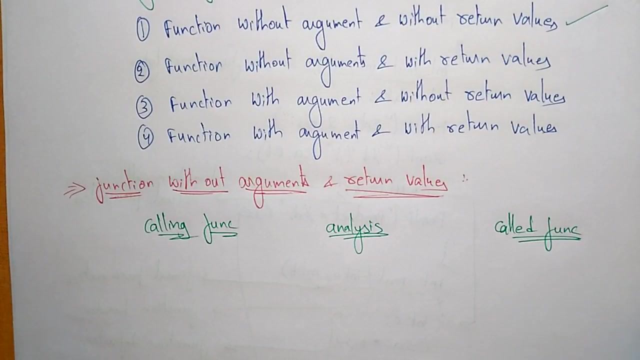 without arguments and return value. Let us see what is this. So here I am taking explaining like this: calling function. I am writing the syntax for this calling function and analysis called function. So in the calling function we use the arguments and return arguments, and called function we will use the return values. 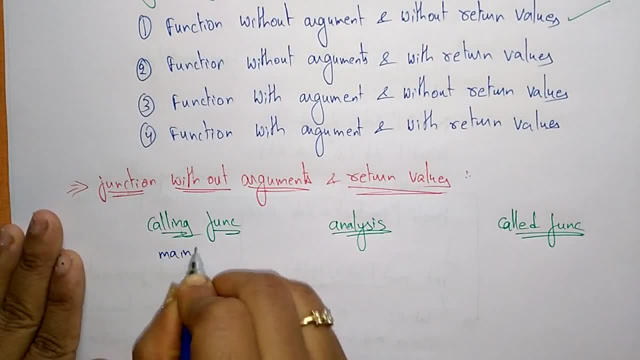 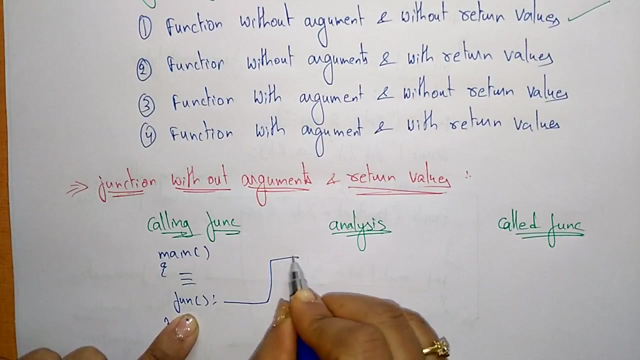 Now let us see how. what is the syntax for this? So here I am writing the main. So in the main, I declare the function and I am calling the function like function. So this is nothing but a function, with no arguments or past. So did you observe here? 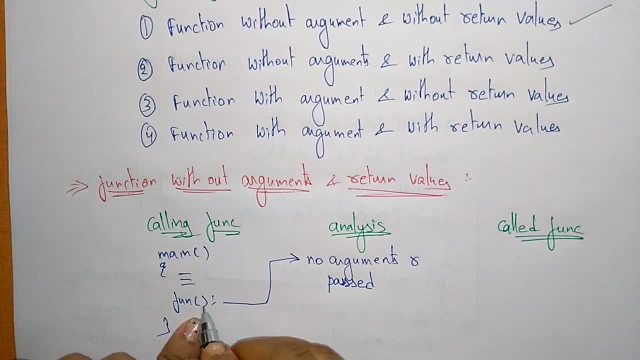 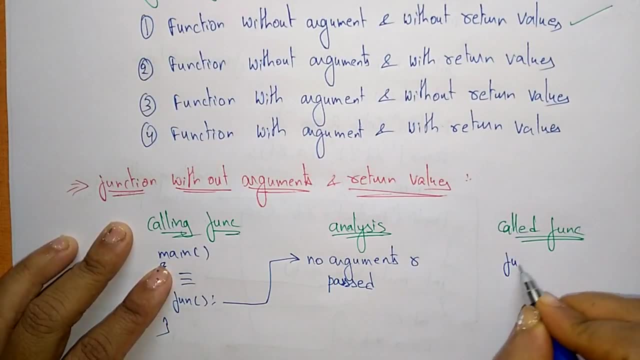 Here, simply the function is there but no arguments are there within the parentheses. So this is a function with no arguments And in the called function function you are just here. this is a calling function and outside the main you are having the called function. 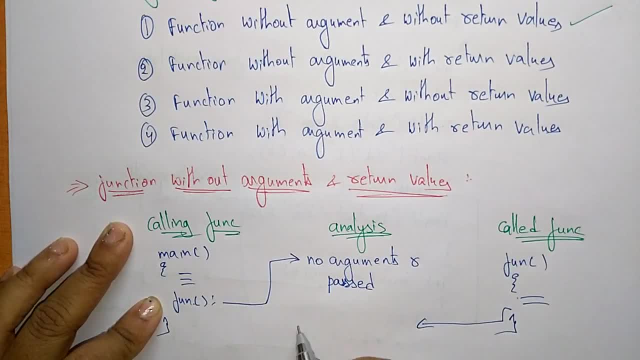 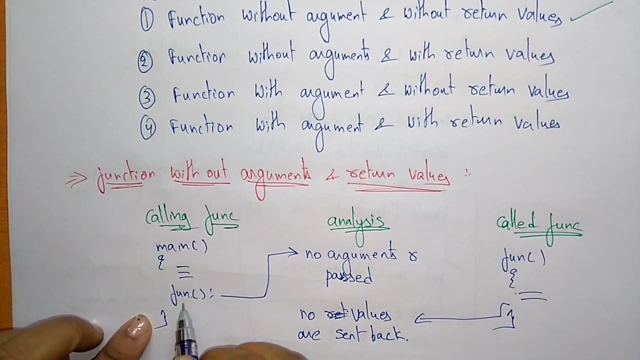 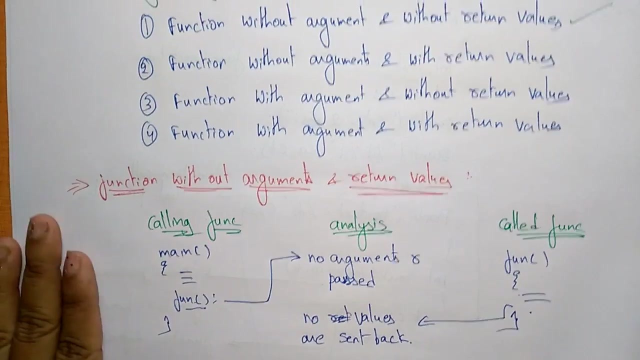 So here a function with no return values. or else you write no values or Sent back, So this is a function with no arguments, A function with no return values. So let us see the example for this I am writing without arguments and without return value. 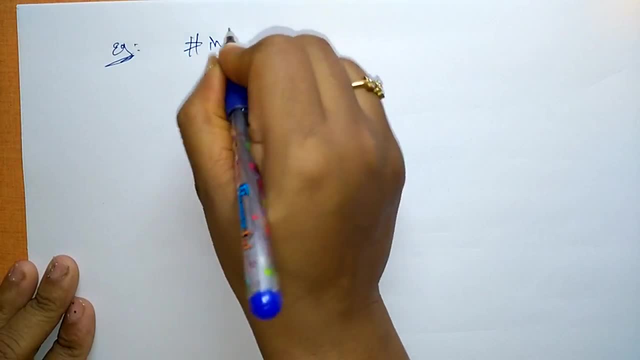 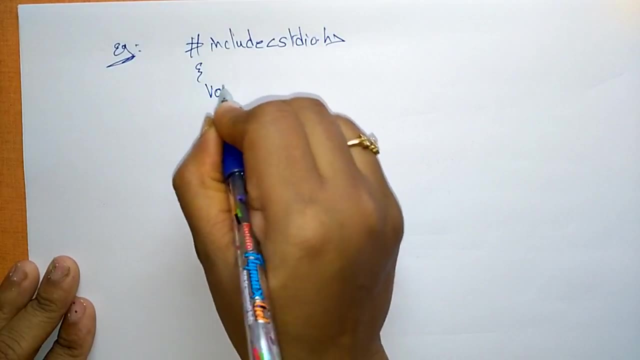 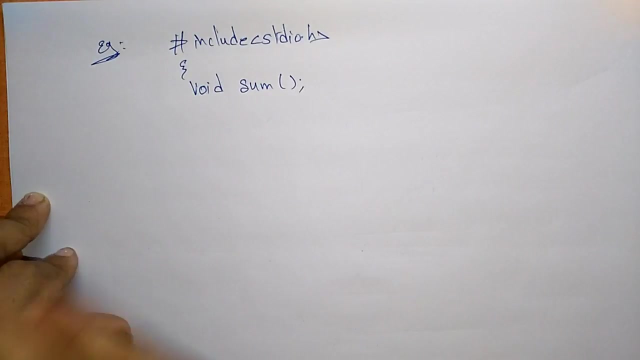 I am writing the program for hash, include stdioh. I am using void, Declaring the function with void return type. What is meant by void? Void means it does not return any value, So here in this example, a function without return value. 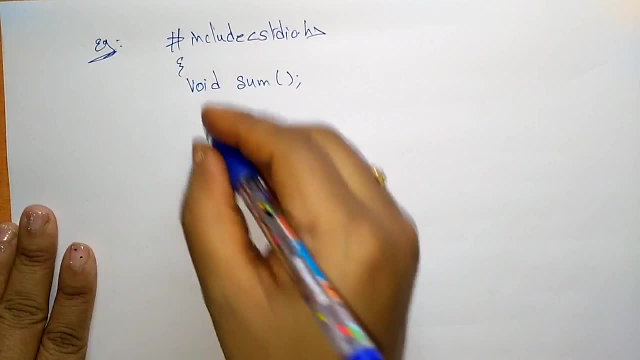 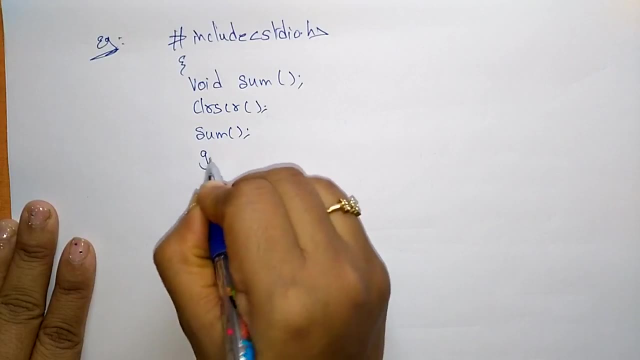 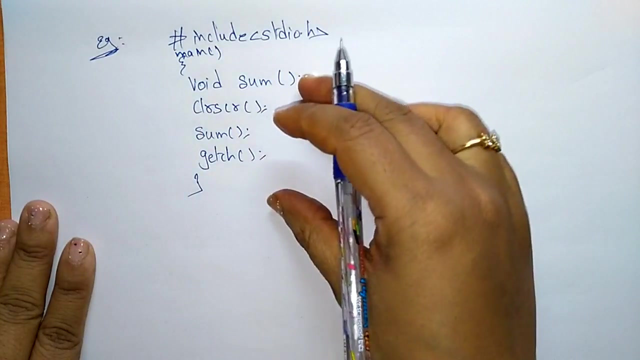 So that is why I mentioned here void. Void does not return any value. Let us see here Again. I am calling, the sum function gets a hash, So this is just a main program. Sorry, here I forgot to write main. So this is the main program. 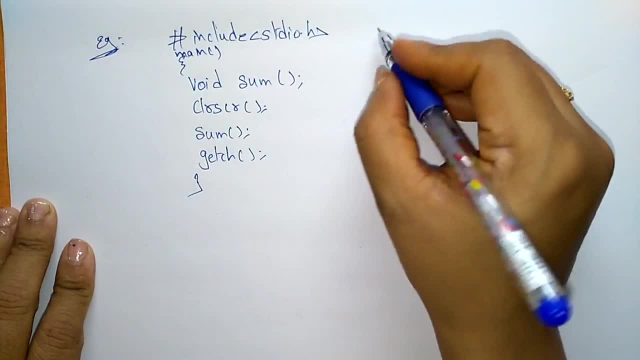 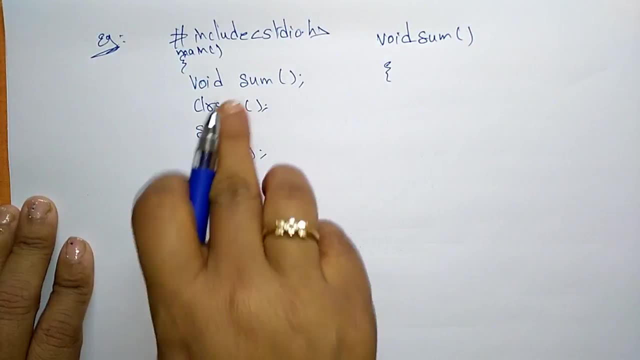 So now I am writing the called function So sum, that is a void sum. I have to write Void sum with no arguments. Did you observe this? Here no arguments are there. So here no arguments in the function. So I am declaring the local variables. 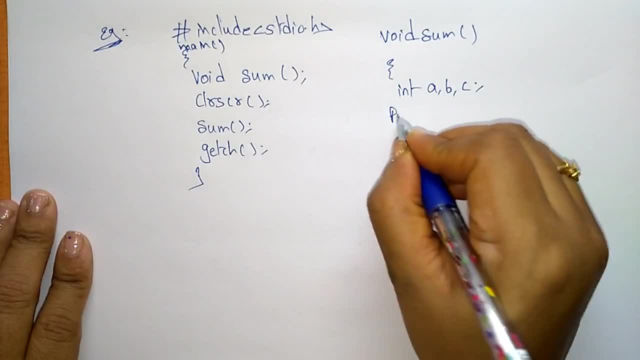 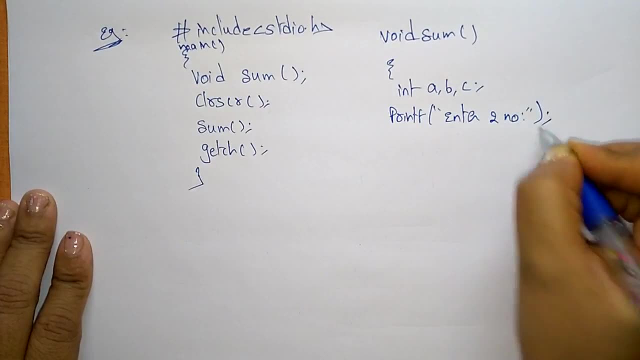 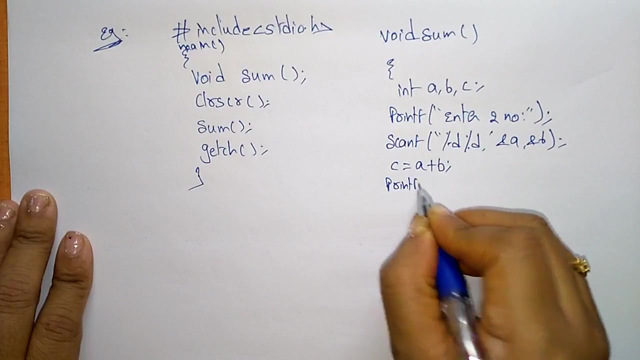 Int a, b, c. Print f. Enter two numbers: Scan f, Amperecent a, amperecent b. Now c is equal to a plus b- And store the c value. Print f. Percentage d, C. Close the function definition. 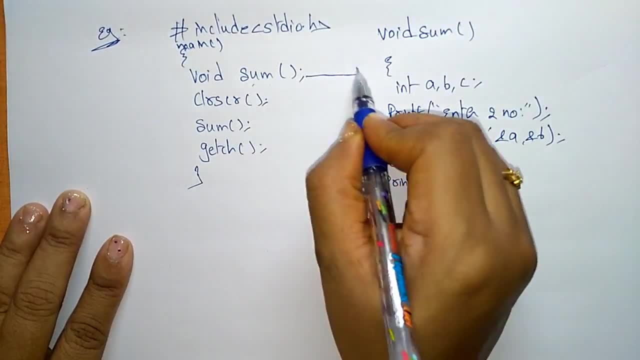 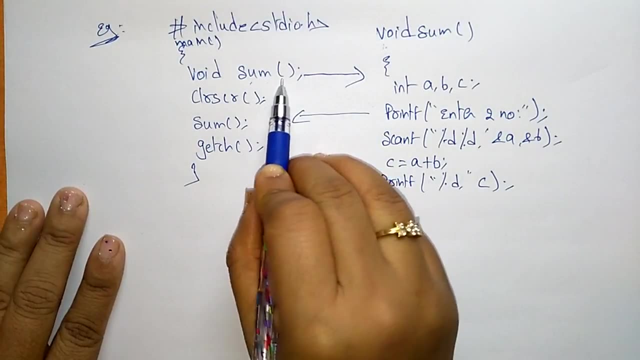 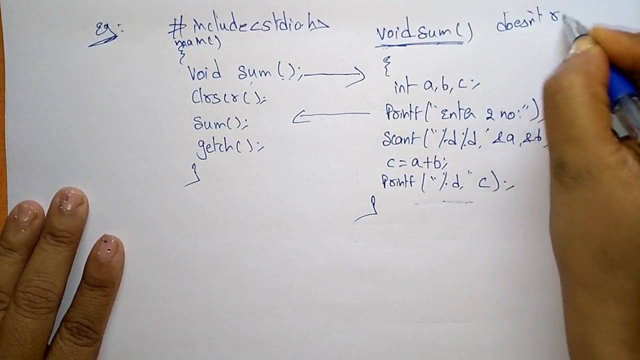 So whenever it is called the control, directly transfer this function. Again it come backs to the main program. So did you observe here This is a function with no arguments and no return value. So void sum means it doesn't return any value. Doesn't return any value. 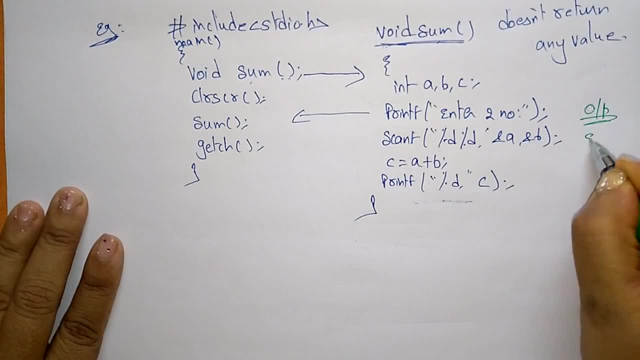 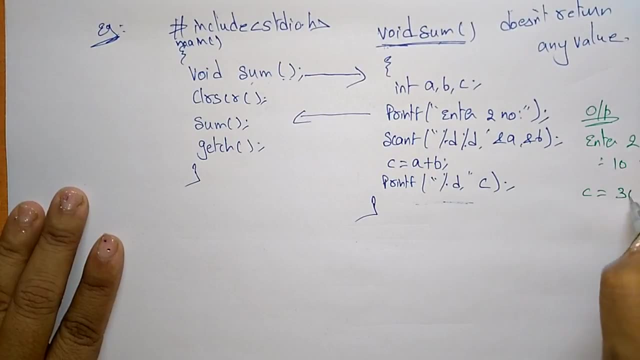 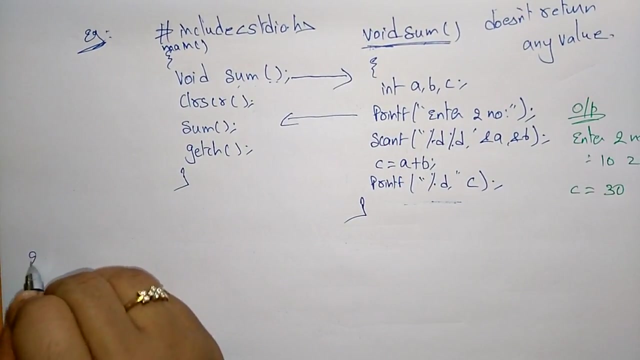 So the output of this program is: Just enter two numbers, That is, 10, 20. I entered Then. now c is equal to 30. So this is a function without arguments and without return values. Now let us see the second category. 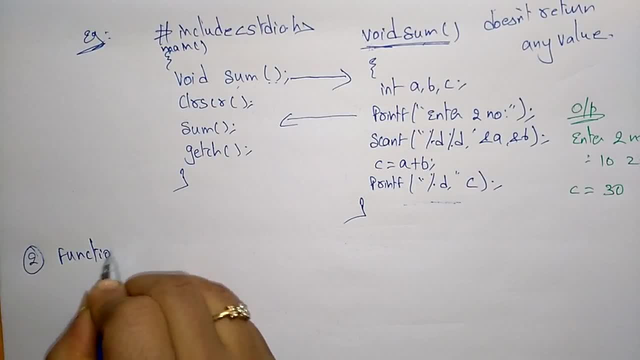 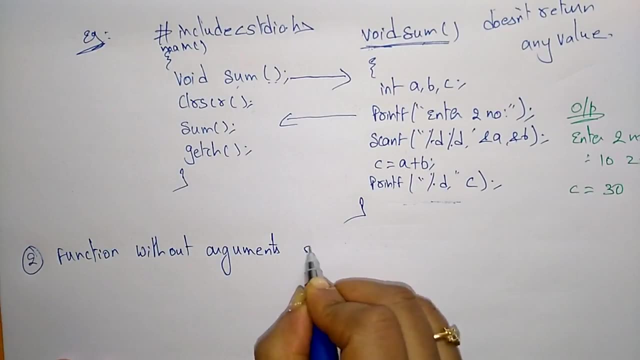 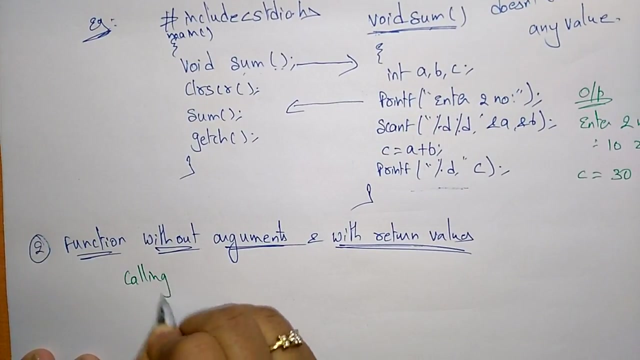 What is the second category Function? Function Without arguments And with return values. So here, no arguments are there, But return values will be there. Now let us see this Calling function Again. I am writing the calling function Analysis. 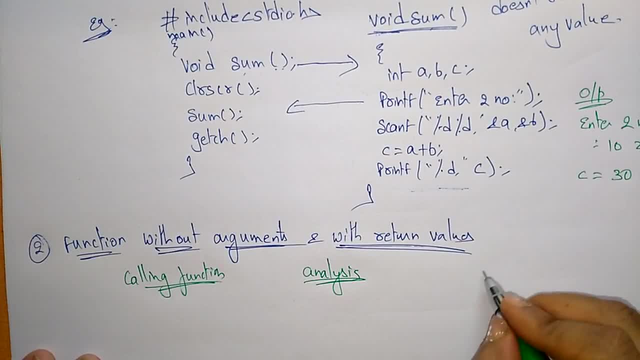 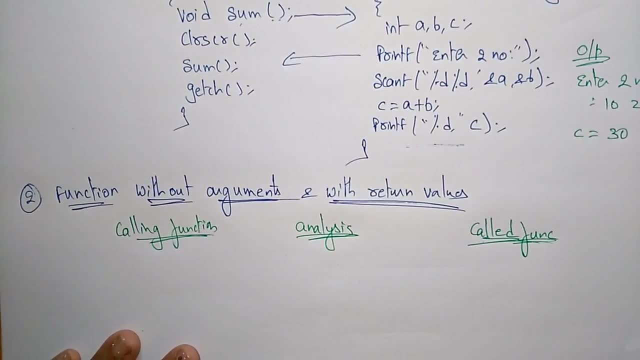 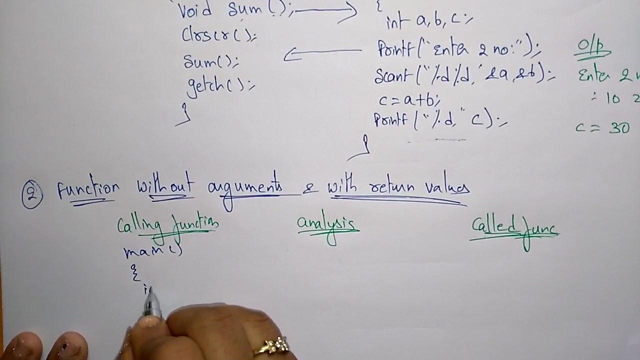 Analysis And called function. Okay, Now write this Main. So here what we have to do: that function without arguments. So declare int c. Now c is equal to You. just call the function with no arguments. So this represents No arguments of. 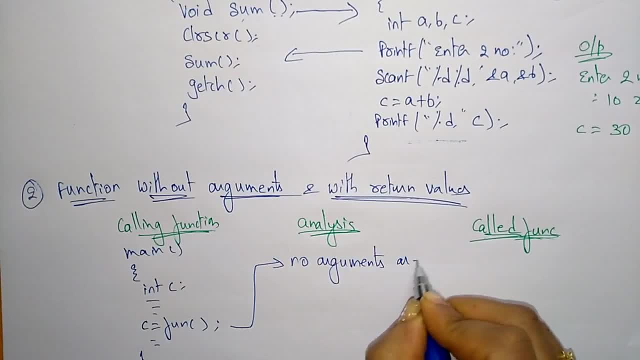 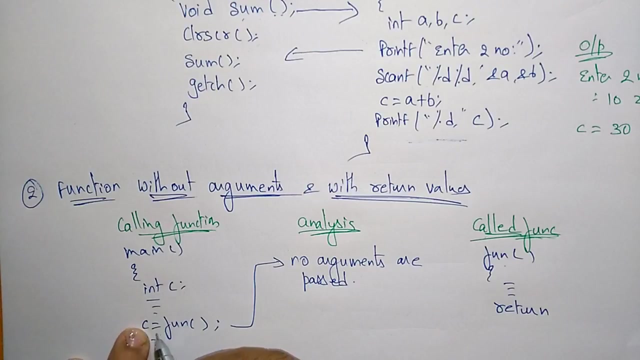 For past, Coming to the called function. So you had to A function with no arguments, But it have some return value. that is a return c. So here I declare c is equal to function, So it is returning some value, Whatever the function you are performing. 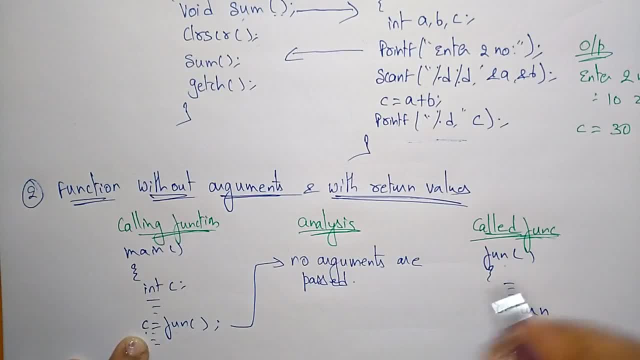 That operation, that result will be stored in the c value, So compulsory it should have a return value that is return c. So here values are sent back. So whatever the value that is in the perform, in the called function, that will be sent back to the main program. 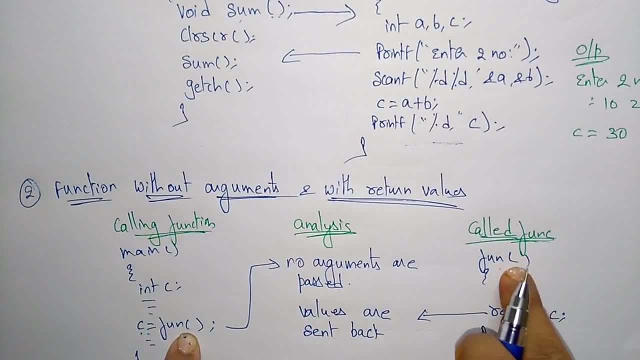 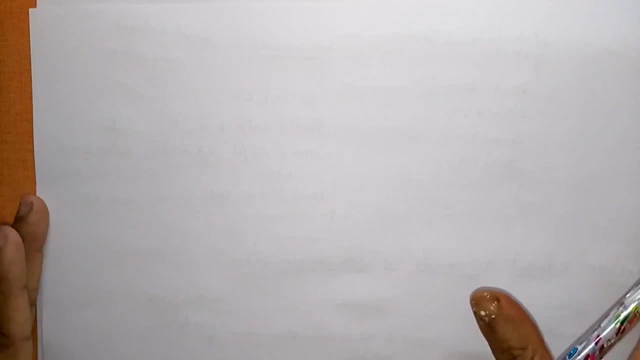 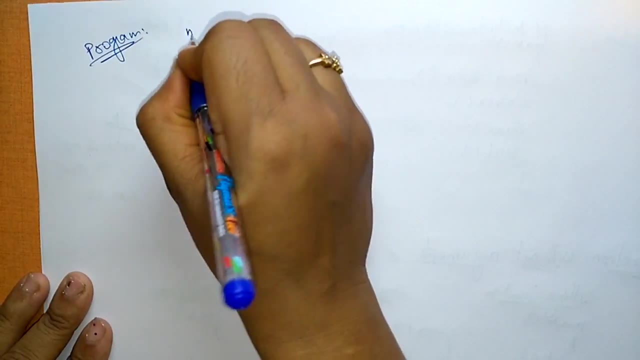 This is function without arguments. So you have seen that without arguments, but with return value. Let us see the program for this, The program for function without arguments and with return value. So just writing the main function, main. Here I am declaring int sum. 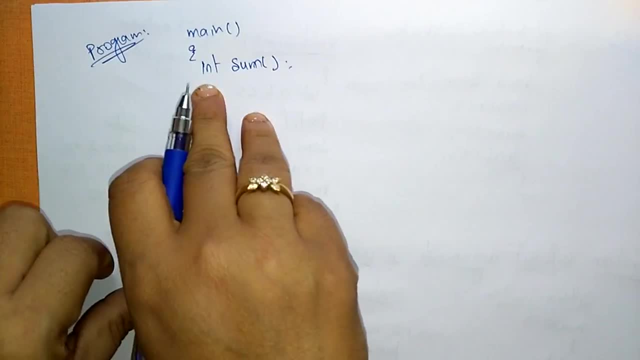 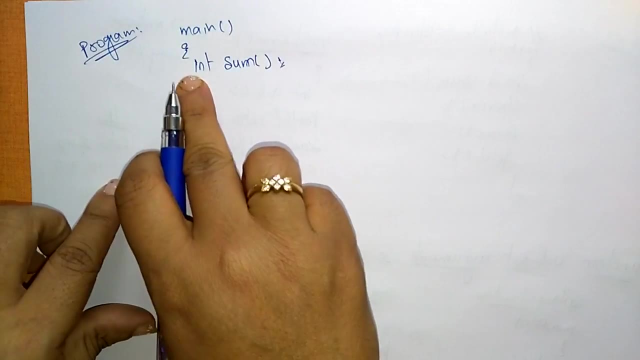 Why I am. in previous example I had used void sum, But here I am using int sum. Void sum means it doesn't return any value. The function: if doesn't return any value, You have to mention it void. But here the function returns a value of integer data type. 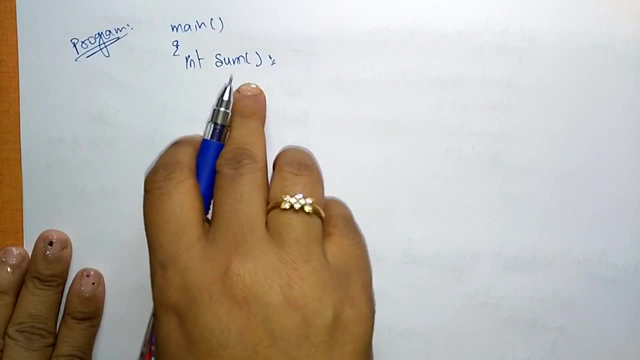 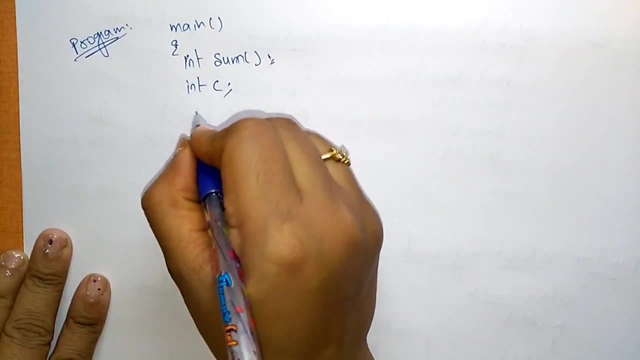 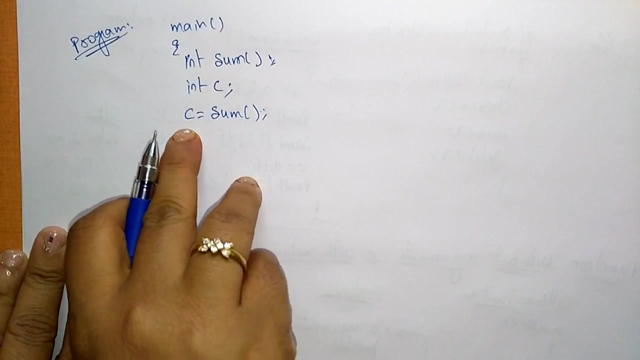 That's why I'm making it as a int, Declaring the function as a int sum. Int sum Int c And c is equal to sum, Because function is returning some value, So that is of integer data type. c is equal to sum. 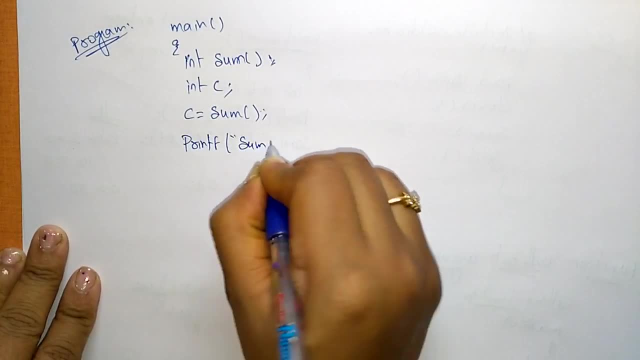 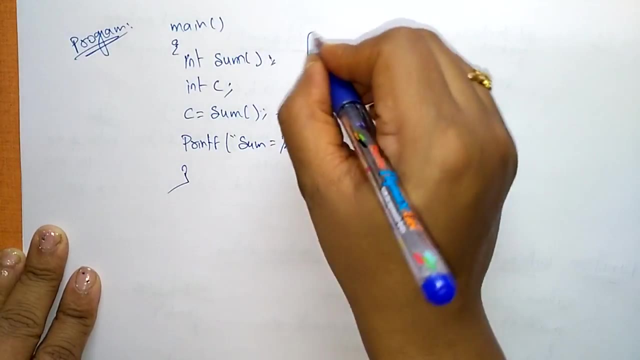 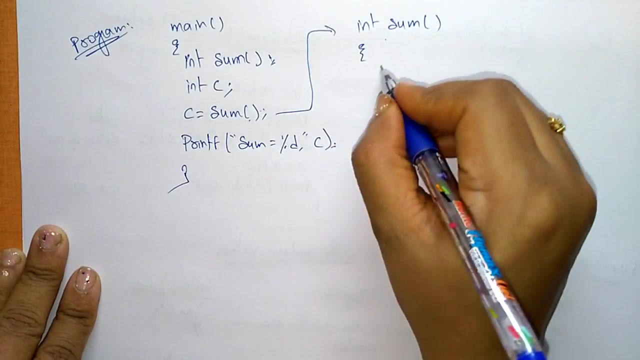 And printf Sum is equal to percentile d, comma, c. Close the main function. Now coming to the call function. So whenever the statement is occurred, It comes, The control jumps to the function And call Int sum. But here did you observe? 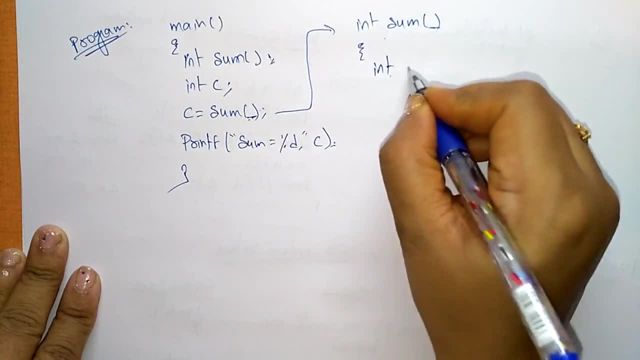 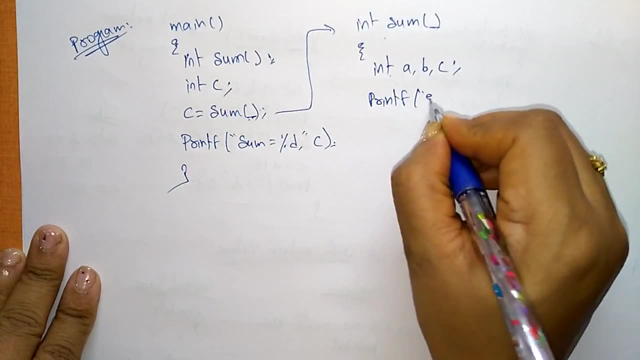 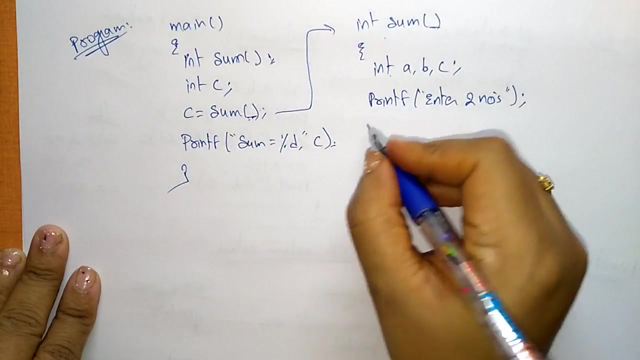 Here no arguments are there. I am declaring local variables. Int a comma, b, comma c. Printf: Enter two numbers For all the functions. I am taking the same example So that you can understand what is the difference between the With arguments and without arguments. 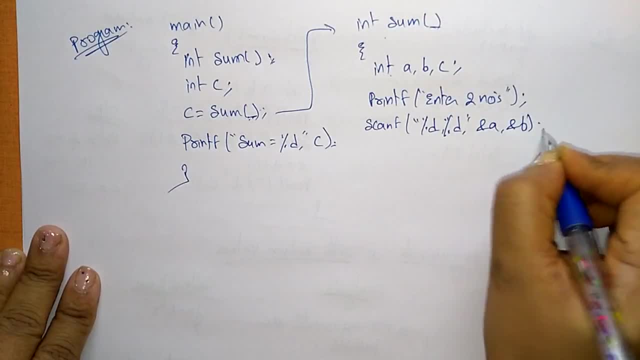 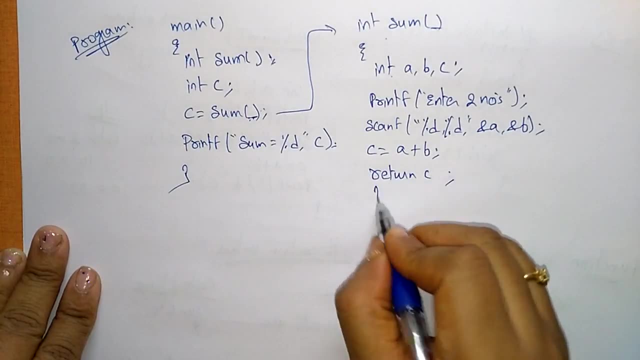 Just simply show all the values. Amperecent a, comma. amperecent b. C is equal to a plus b. Now I am returning the value return c. So whenever I mentioned returns, Close the function call. So whenever it is there. 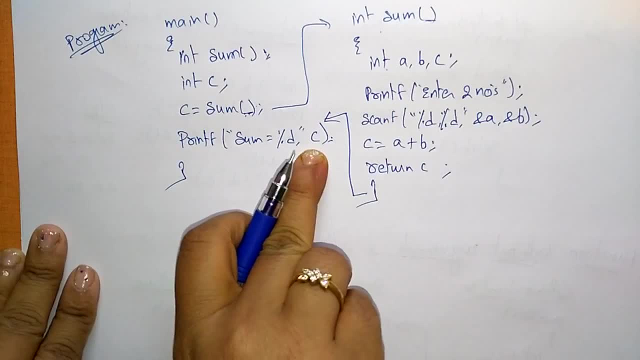 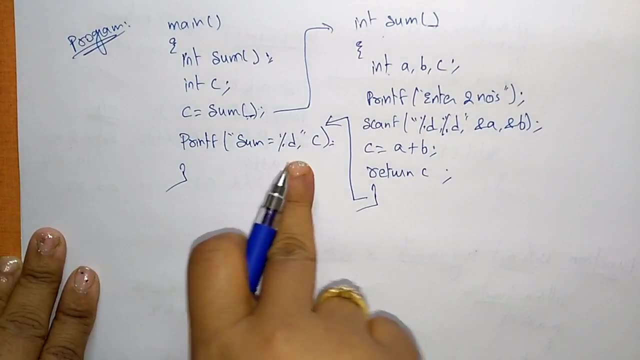 Again, the control jumps to this here And prints the c value c is equal to some, So it is returning the value C and stored in the c That has to be print on this screen. Then what will be the output for this? 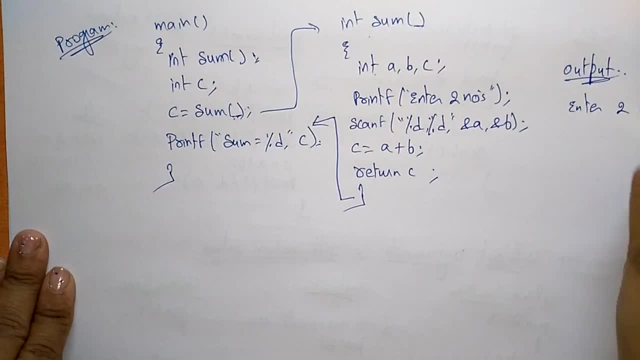 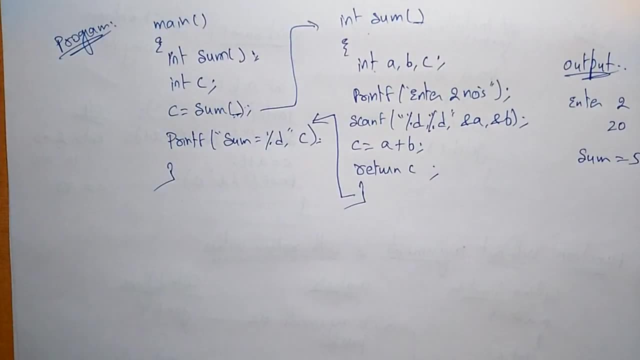 Just enter two numbers, 20, 30, and sum is equal to 50.. So this is about the function without arguments and with return value. Now let us see the third one. So what is the third category? Coming to the third category, 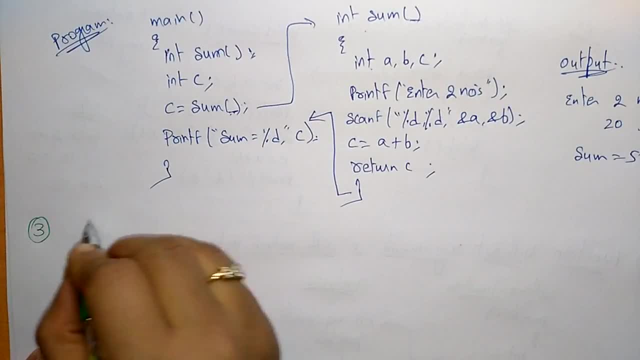 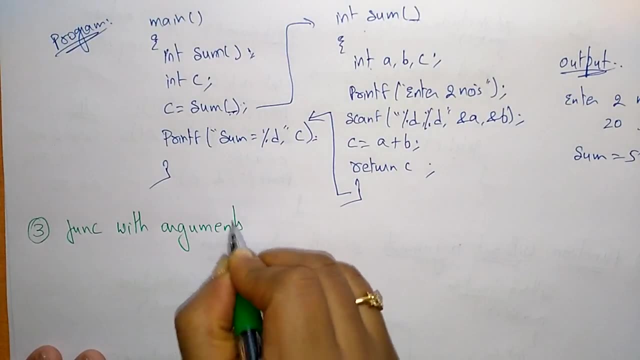 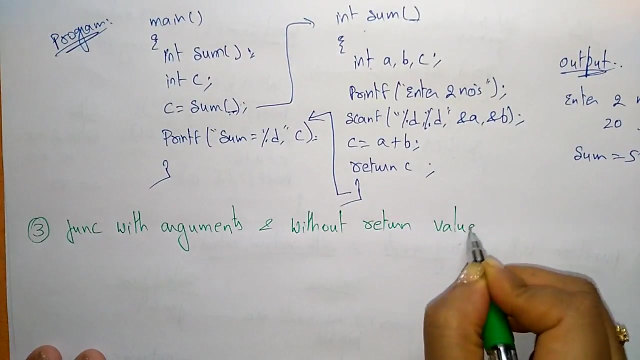 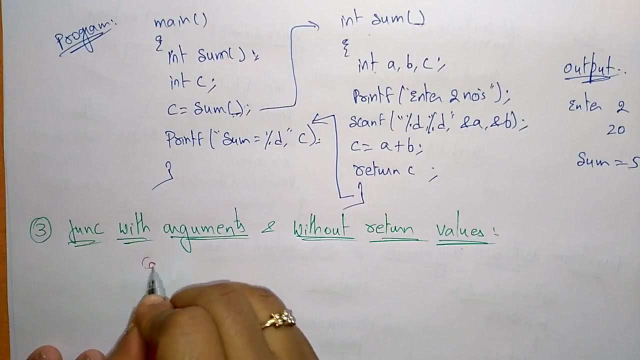 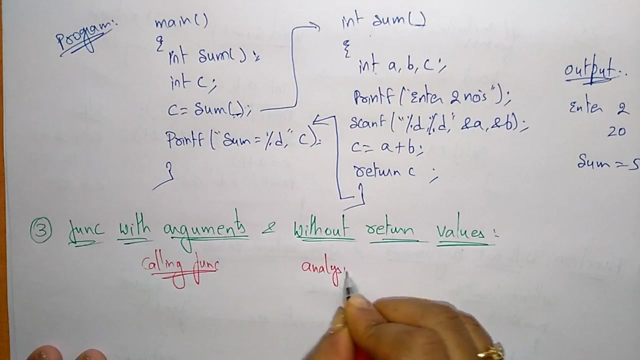 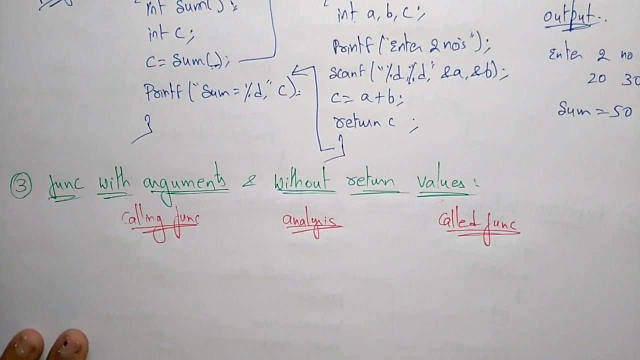 The third category is function with arguments and without return values, Without return values. So third category is function with arguments and without return values. So again, I am writing the calling function definition and analysis And call function. Let me write this: 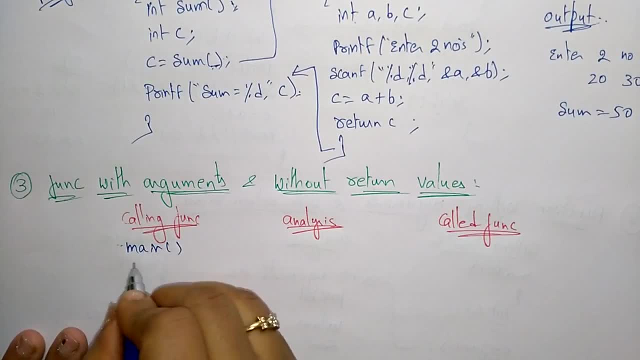 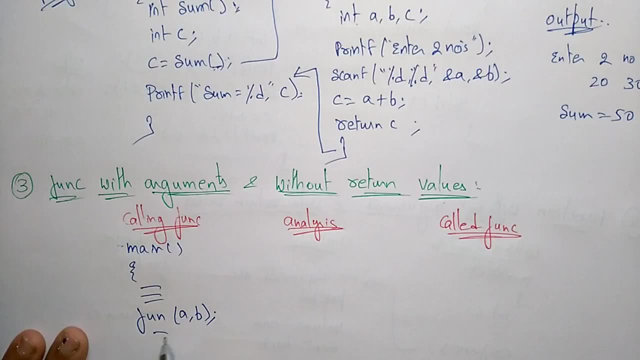 So main here the function has with arguments. So declare the function with arguments. Function a, comma b. So this represents arguments are passed. So two arguments are passed. So two arguments are passed here. Function with arguments Now in the call function. 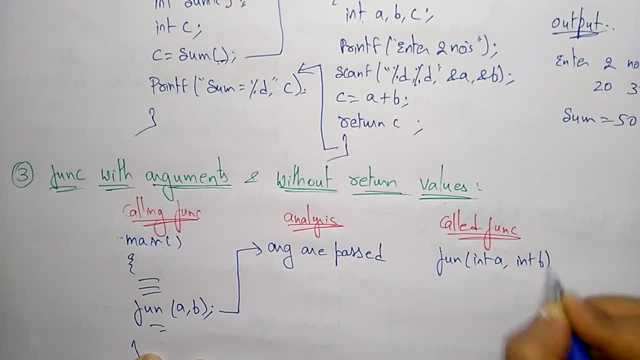 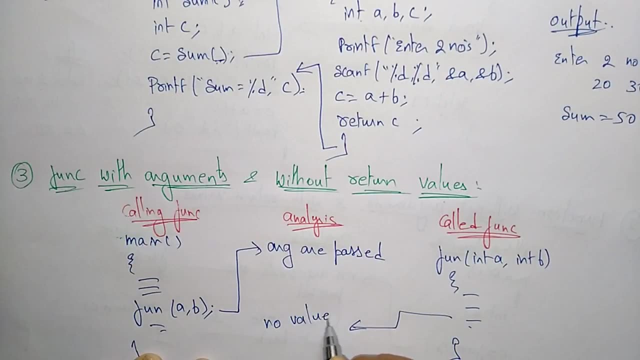 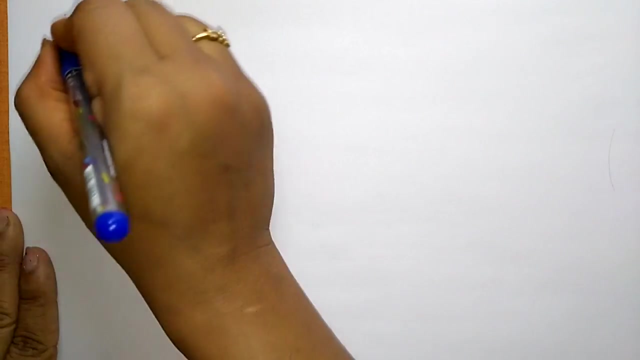 Function: int a, comma, int b: Here no return value is there, No values are sent back. So this with arguments and without return values. Now let us see the program for this, The program for function with arguments And without return values. 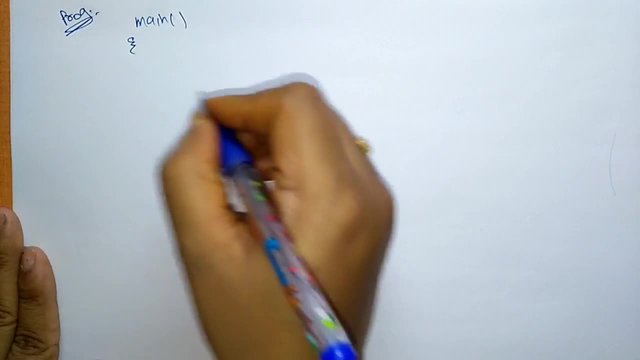 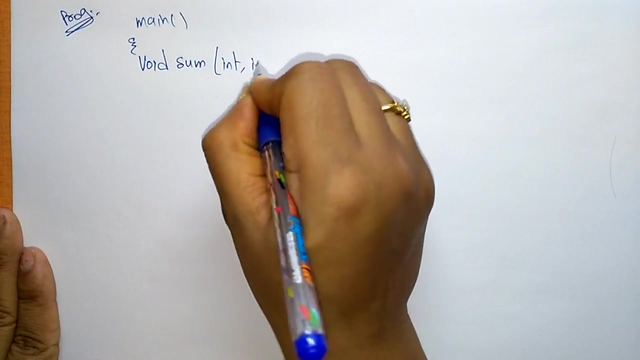 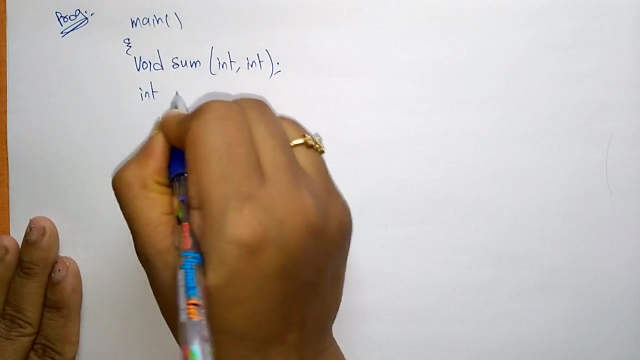 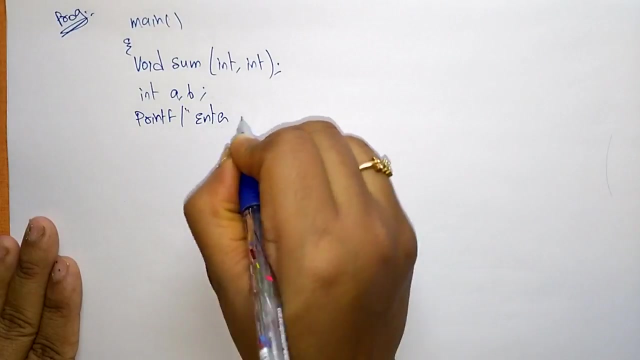 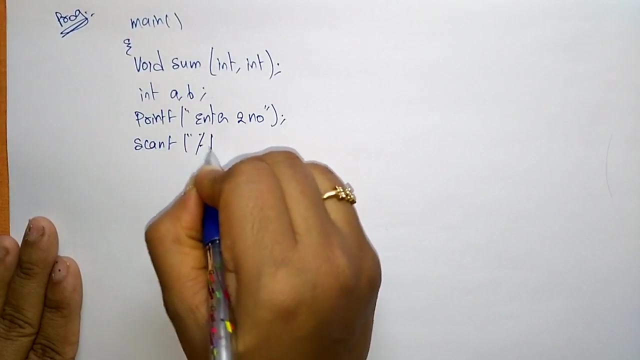 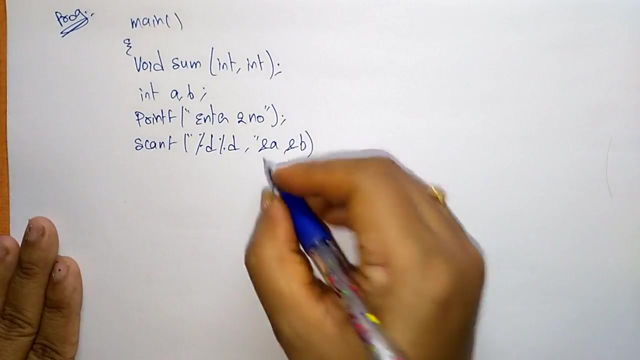 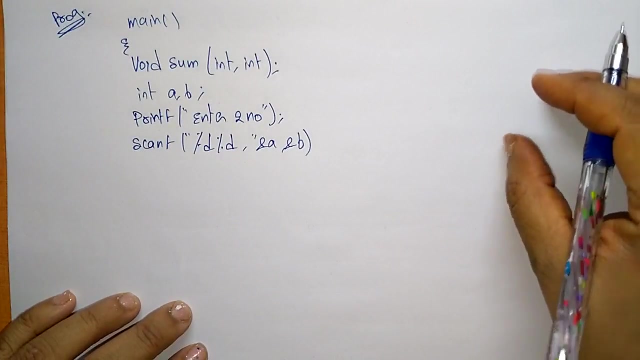 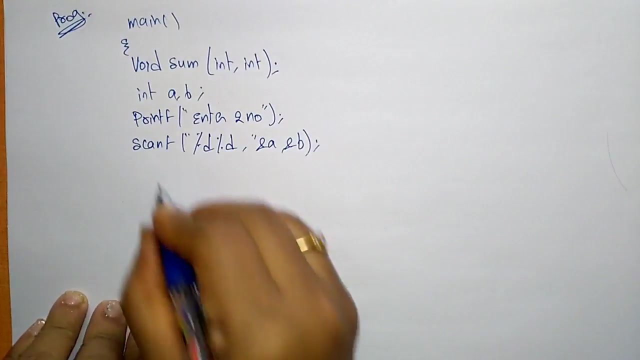 So writing the main function directly Main, So void sum, Because it doesn't return any value. So the void sum With arguments. This is a function declaration: Int a comma b, Print f, Enter two numbers. So here we are passing the arguments. that's why in the main program itself we are declaring, we are entering the values. so if argument, if the function doesn't pass any arguments, you have to declare those variables and you have to print the values in the function. call itself, called function itself, now calling some of a comma b. 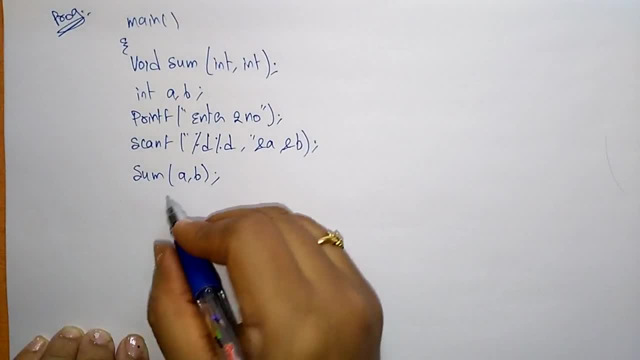 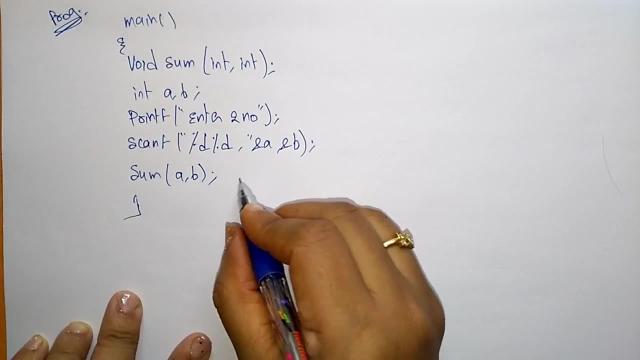 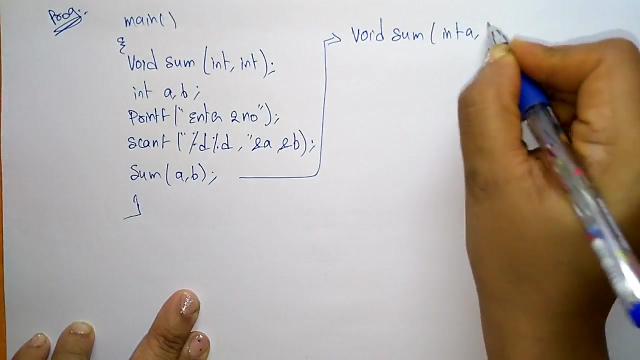 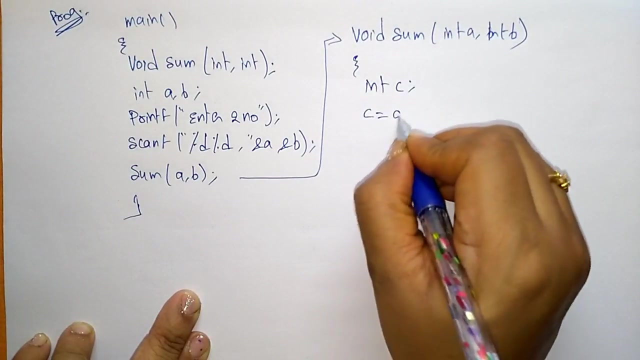 We are not assigning this sum to a Any return value, because this is function with arguments and without return values. Close the main. So whenever this is there, the control jumps to the Void sum. Int a, comma, Int b. Now I'm taking in c as a variable- c is equal to a plus b- and printing those value. 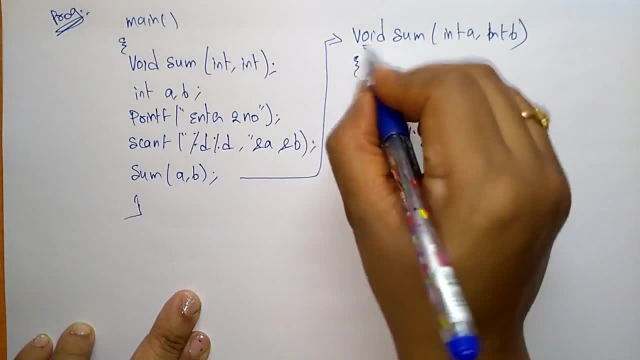 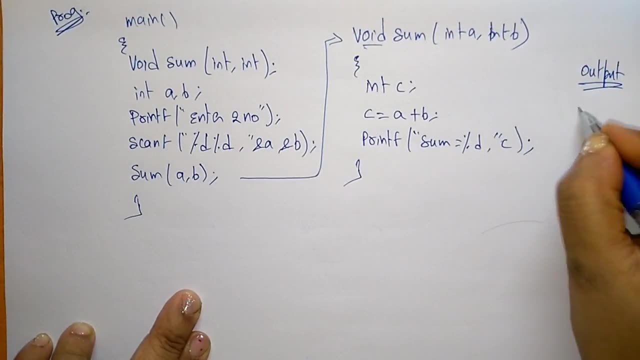 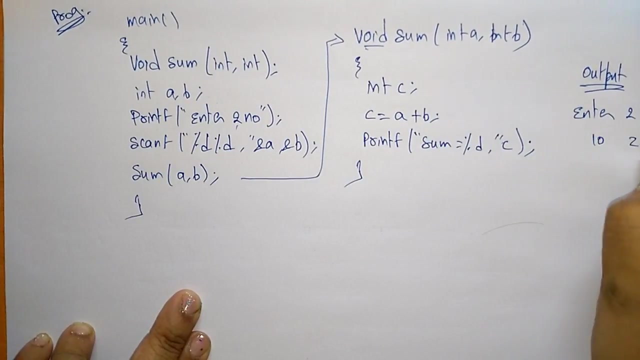 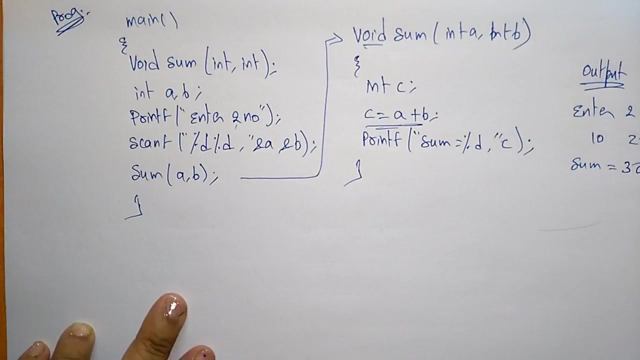 Here the function doesn't Return any value, because this is voids Some. Now the output is: Enter two numbers. So here two numbers: Ten, twenty. now the sum is equal to A plus b, that is thirty. So this is a function with arguments and without return values. now coming to the last category, that is a fourth category. 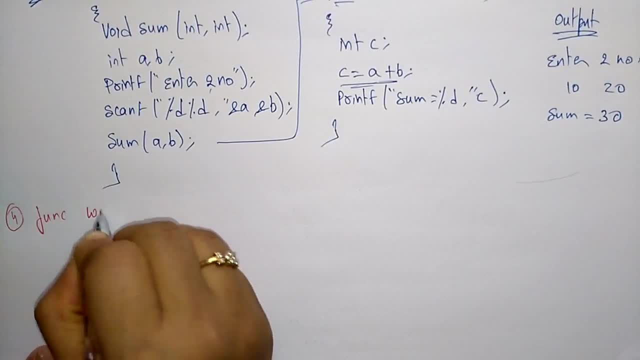 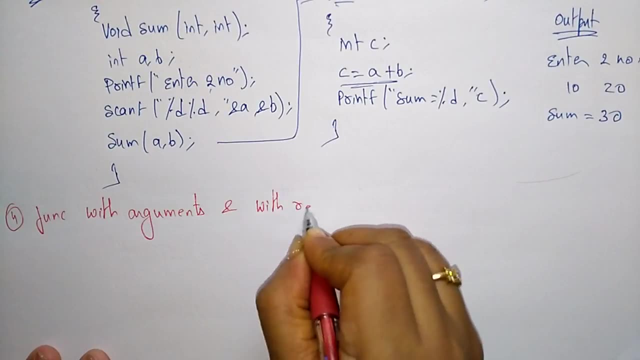 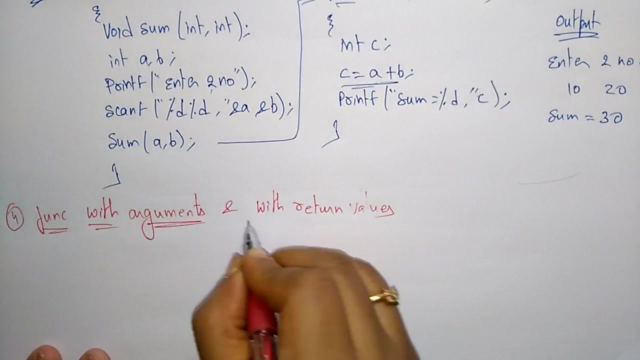 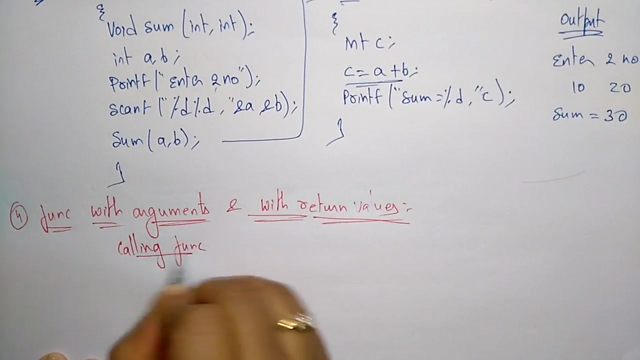 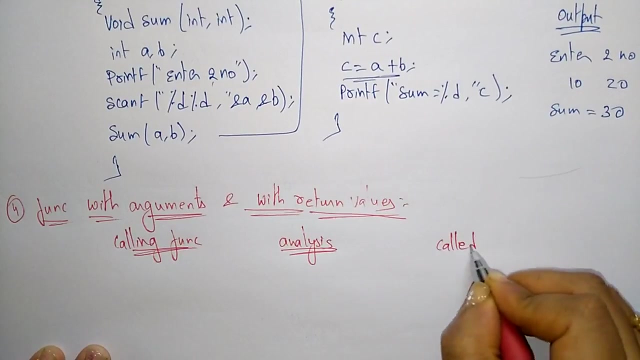 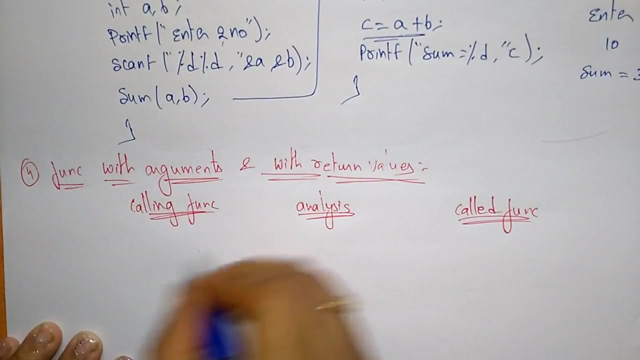 So function With arguments And with return values, function with arguments and with return Values. So let us see So the categories of calling function, Analysis and call function. now coming to this, here main into C. so here function with: 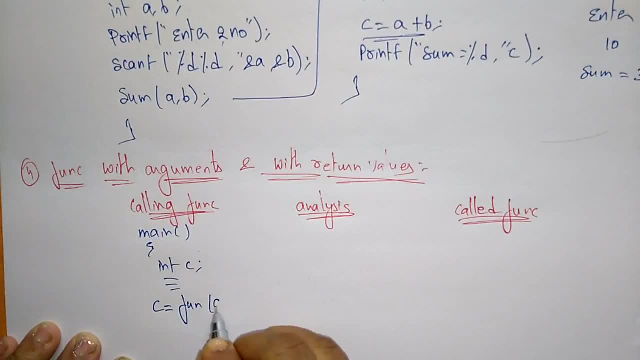 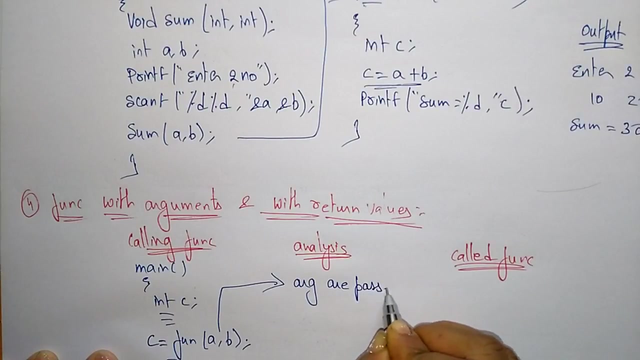 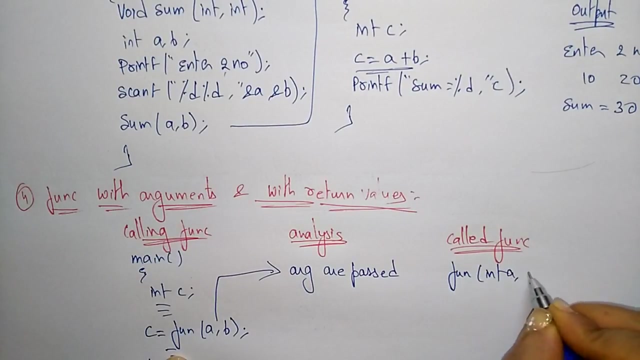 return value at the same function with argument. so this is the return value and this is the function with arguments. so this represent arguments or past. now coming to the called function. so in the call function function, int a, comma, int B, function with arguments, and the same weights have the return value C. so this: 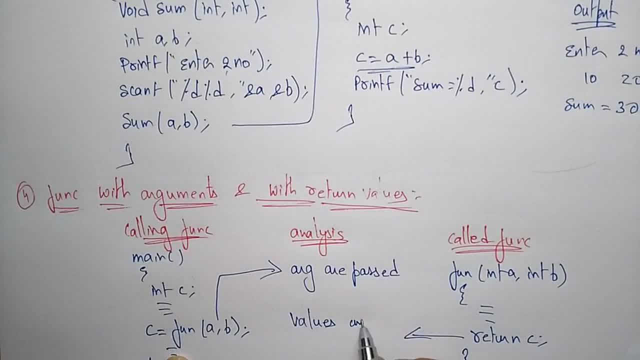 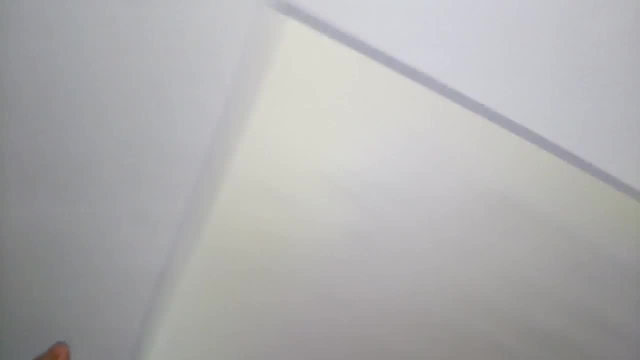 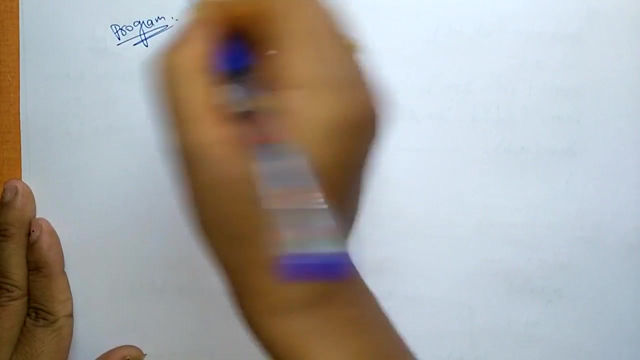 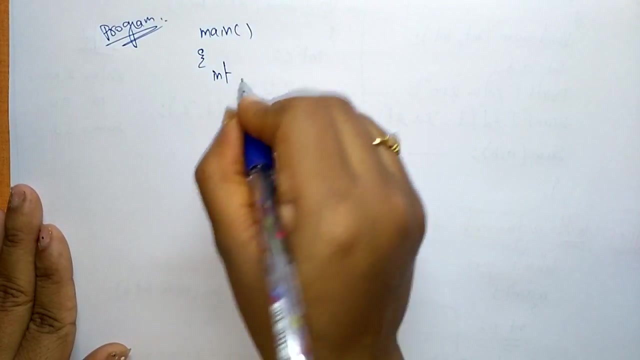 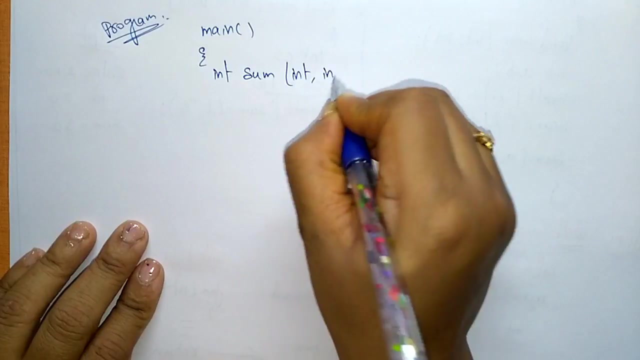 represents values or sent back. so this is function with arguments and with return values. now let us see the simple program for this program. so write the main program, main function. so here I'm declaring the function name with data type into- because it written somewhere- integer, data type, value and arguments to arguments. so this is the 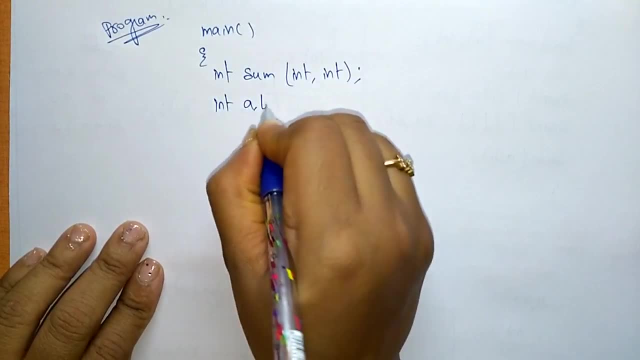 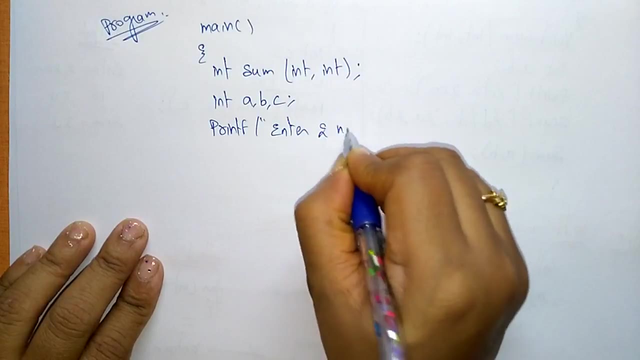 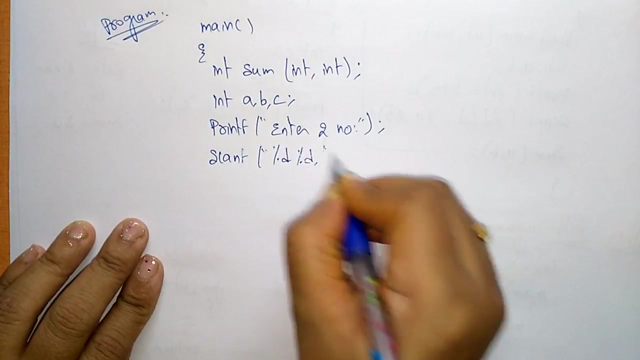 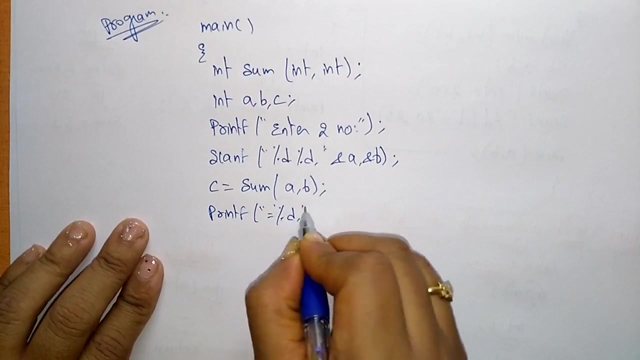 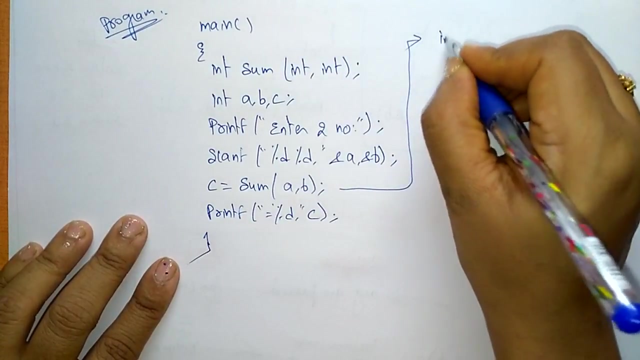 function declaration. int a comma B, comma C printer and two numbers: scan F and present a comma person. be C is equal to some of a comma B. so this is a calling function printer. see close the main function. so whenever the function call is appear, the control jumps to this call function in some. here i'm declaring that this is a function.